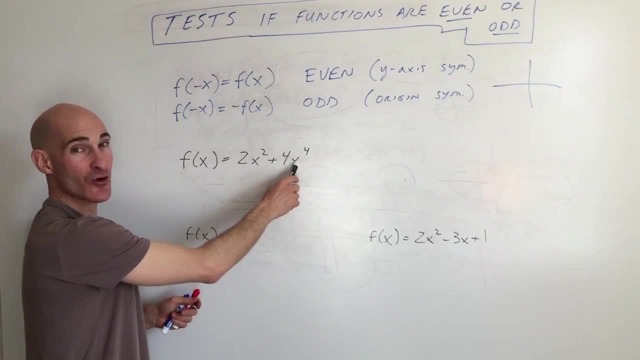 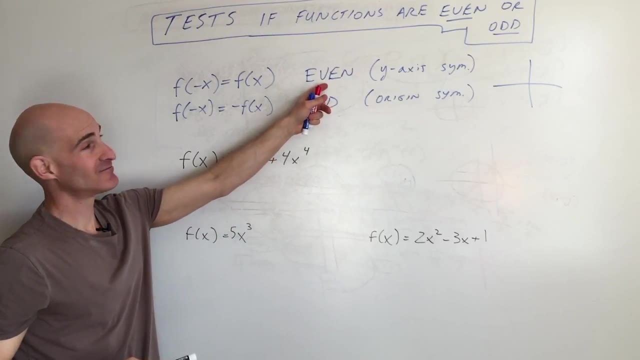 parentheses- negative x. you're going to put that in place of x on the right. If you get back the original function, exactly like how the original function is, that tells you that it's even If you replace x with negative x and you get the same function back, the same terms. 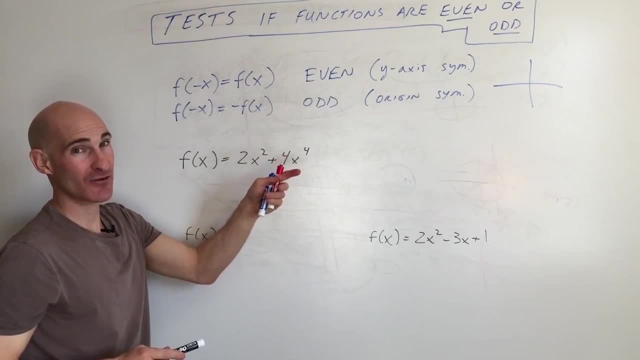 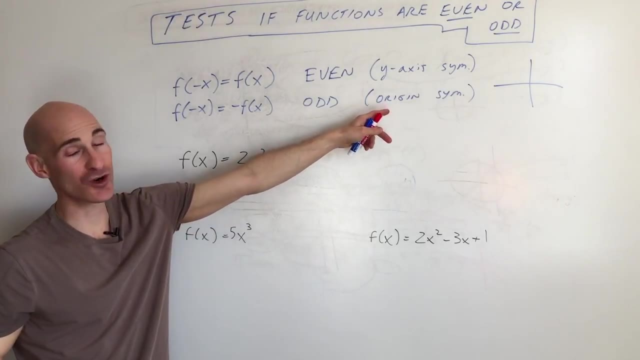 but all the signs are the opposite. okay, if they're positive, they're negative, they're negative, they're positive, they're flipped. that tells you that it's odd And that it is a rotation about the origin. okay, so I'll show you some examples here. let's take a. 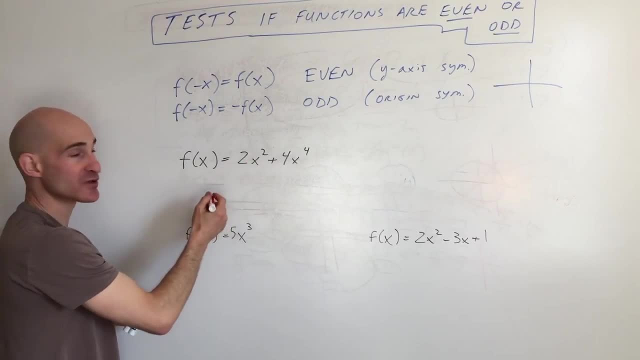 look at this example: f of x equals 2x squared plus 4x to the fourth. if we put negative x in, okay, we're going to get 2 negative x, the quantity squared plus 4 times negative x to the fourth power. a negative to an even power is a positive, so we're just going to get back 2x squared. 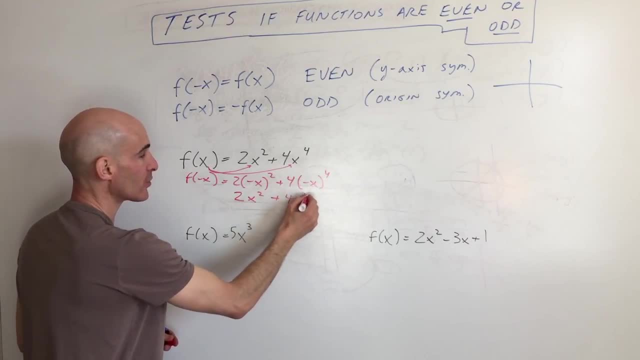 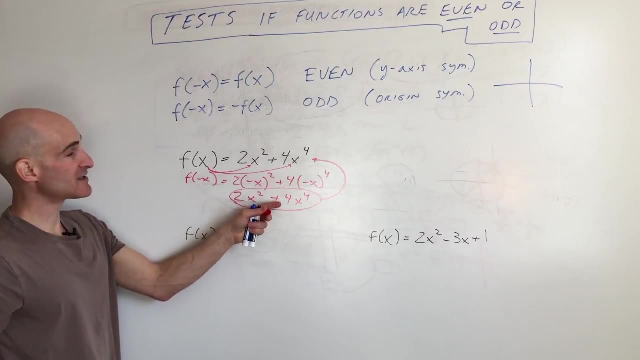 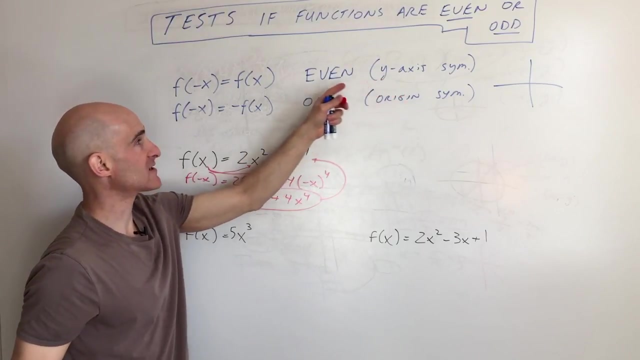 a negative to an even power, we're going to get a positive x to the fourth. you can see we're getting back the original equation exactly how the original one was. so that tells you that this graph is even okay. it has even symmetry and it's a reflection over the y-axis, but we just call this even so. 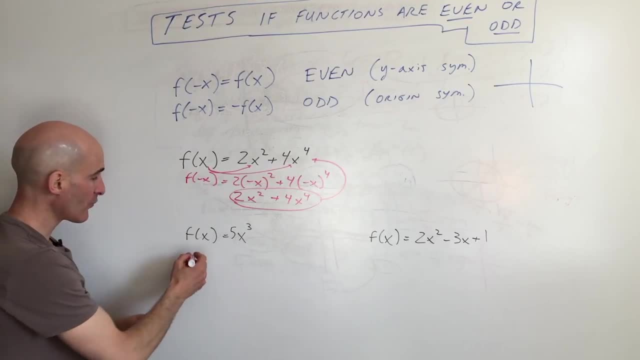 this is the test, for even you're substituting a negative x. same thing over here. we're going to put negative x in place of x here on the right, and if we do that we get a negative to an odd power which is going to be negative. so this works out to be negative 5x cubed. it's exactly. 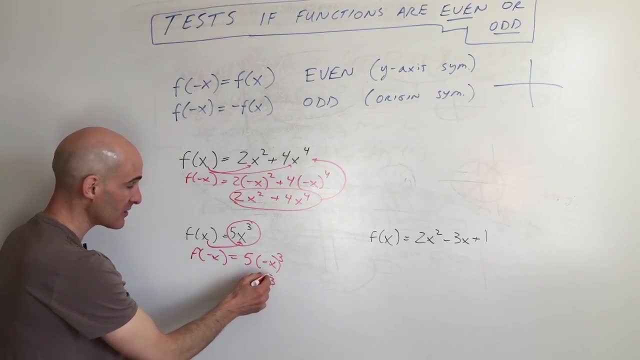 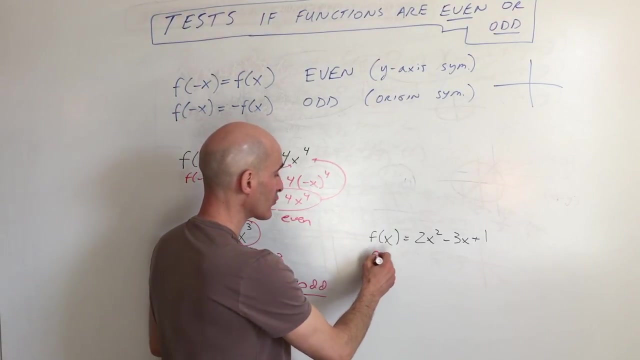 like the original function, but the sign here is the opposite. so that tells us that this is odd. okay, so we have, even for this one, odd for this one. okay, now, over here we're going to do the same thing. we're going to put negative x in place of x on the right side of the equation. so 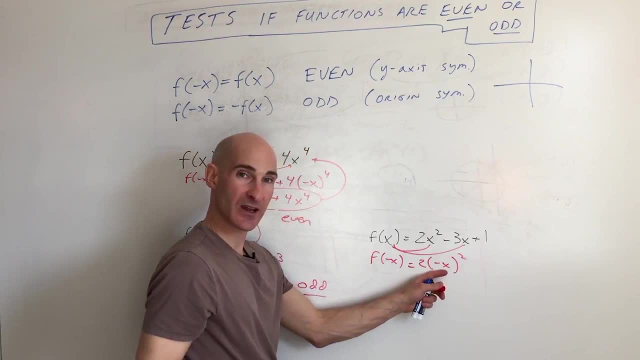 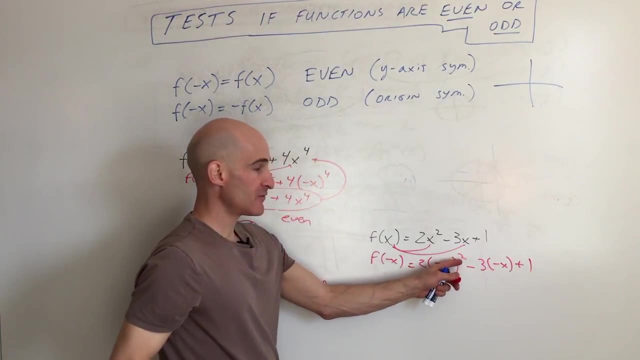 that gives us 2 negative x squared. negative x squared. Notice I put the negative x when I substitute in parentheses, so I take it as a whole. okay, as a group. A negative to an even power is positive. so that's giving us 2x squared.